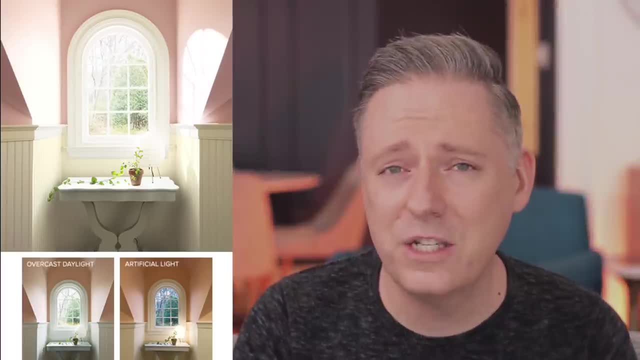 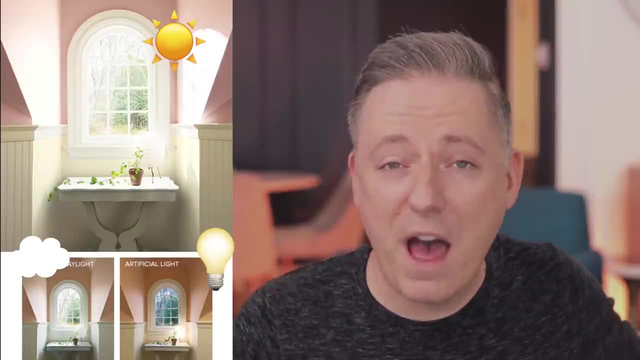 is the importance of light on color. Light completely changes color. I cannot state that strongly enough. So a paint that works in my living room is not necessarily what's going to work in my bathroom. It will appear very different. It'll appear completely different in your living. 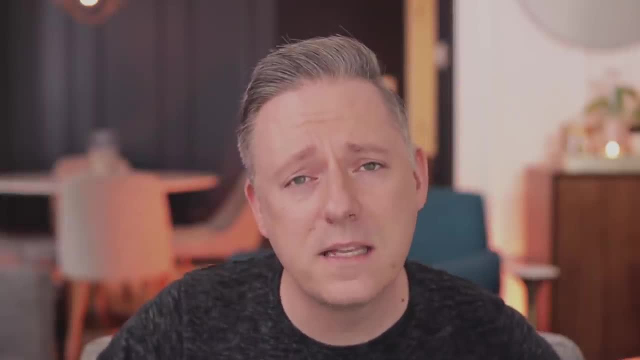 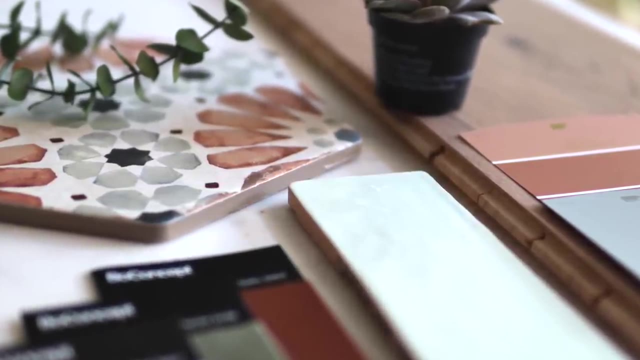 room, It will always look different. So my advice to you on this is to always get samples of paint or fabric swatches or flooring samples or whatever you need, to make sure that it's all going to work together in the rest of the color palette. Get it in your home. See what it looks like in your 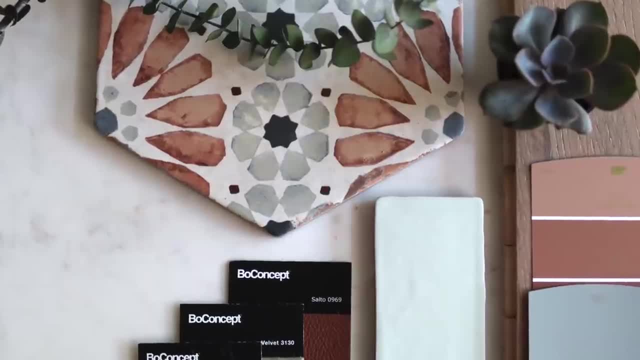 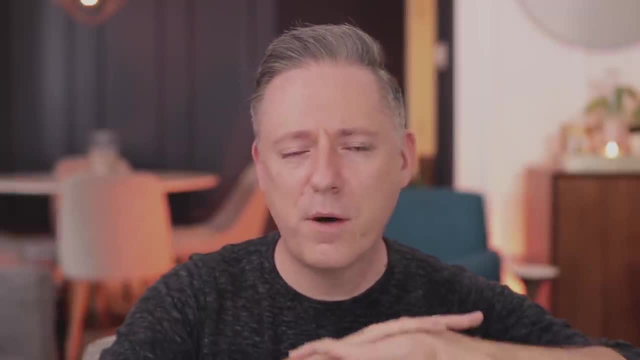 lighting, because it will look different than it does on the shop. It'll look different than it does here in my apartment. So that's my disclaimer. It's just always making sure you get samples, because it will change everything that I talk about for the rest of. 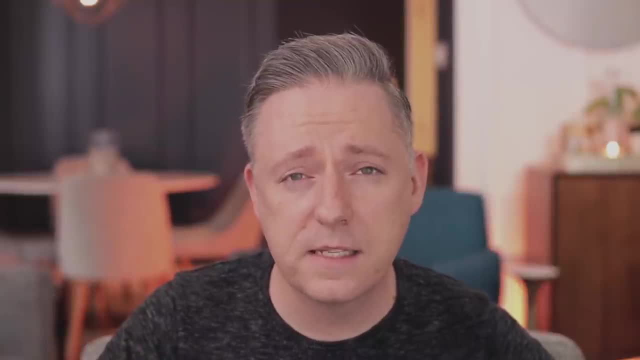 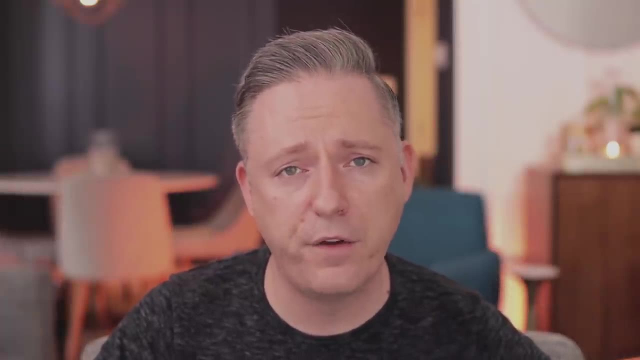 this video. So let's get that out of the way, Okay. So let's do some basics of color theory. I promise it'll be interesting and I promise you're going to learn something from it, and it will really, really, really help you create a beautiful color palette for your home. So this 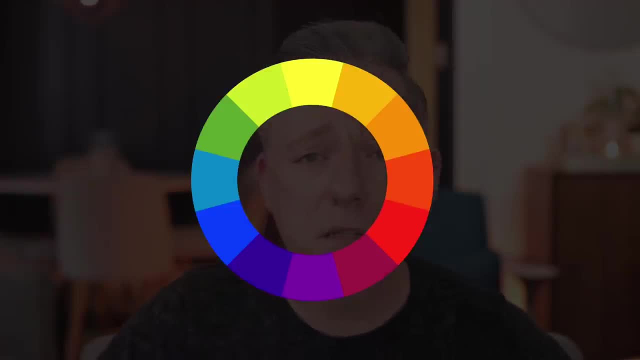 is the old color wheel. Okay, We remember this from grade school. Okay, So first let's talk about color temperature. So there are cool colors and then there are warm colors on the color wheel, right, So the cool ones are blues and purples, greens, And then, on the warm side, you've got your. 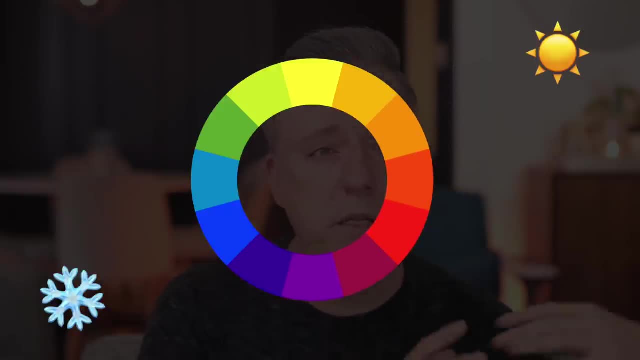 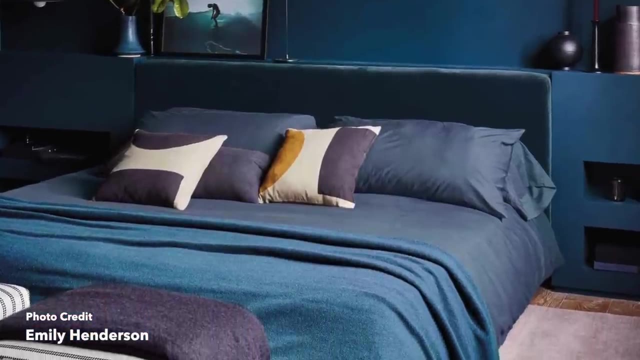 reds and your yellows. The cooler color tones typically create a really soothing or sophisticated atmosphere in your space. Those can be really great for bedrooms, Cause you know you're probably going to be sleeping there. You great for bathrooms, but those warmer spaces can be. 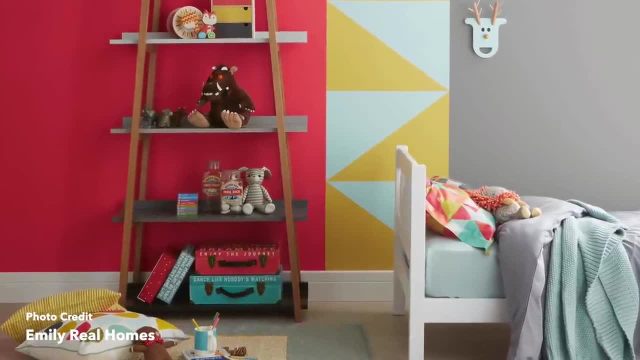 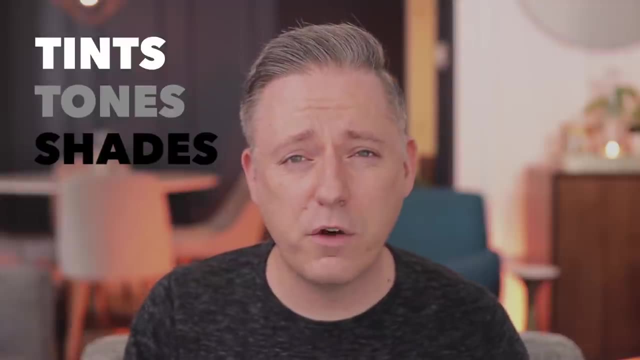 really energizing. They can be great for offices or kids' playrooms. Okay, So now let's talk about something that I think really trips people up a lot, which is tints, tones and shades, Cause I feel like a lot of you have probably heard these words, but you don't necessarily like super. 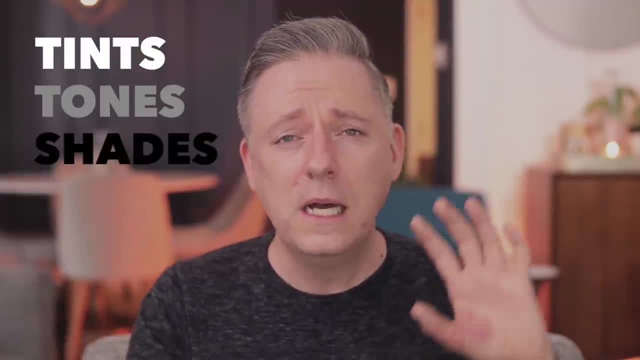 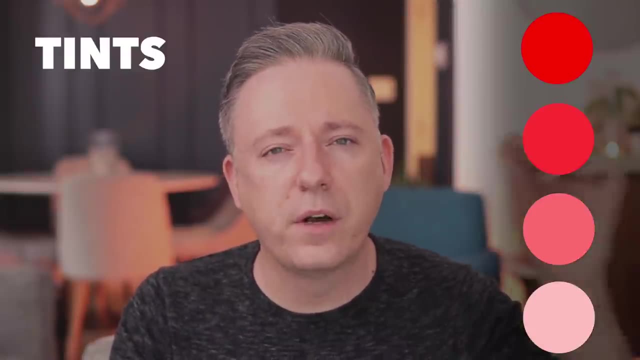 understand what they mean And that's okay because we're going to talk about them right here. So tint is just looking at all those different colors that exist on the outside of that color wheel And it's adding white to those different colors. So if you take something, 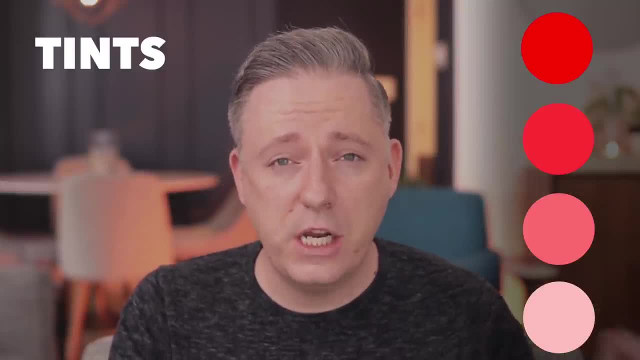 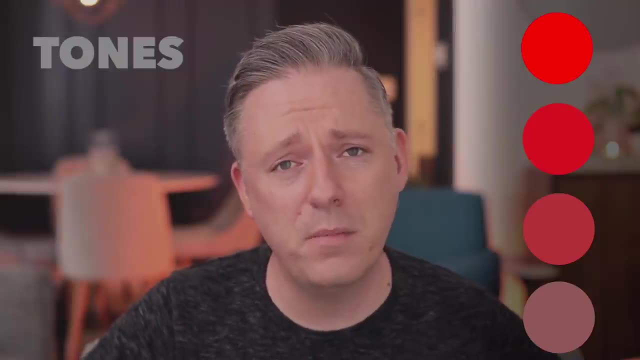 like a color red and you add a lot of white to it. it's going to change it and it's going to become pink Tones just mean that you take those colors or those hues that are on the outside of the color wheel and you add gray to them. So typically, what happens when you add gray to some of these colors? 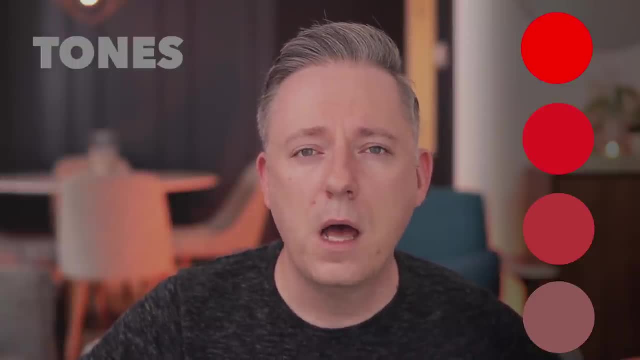 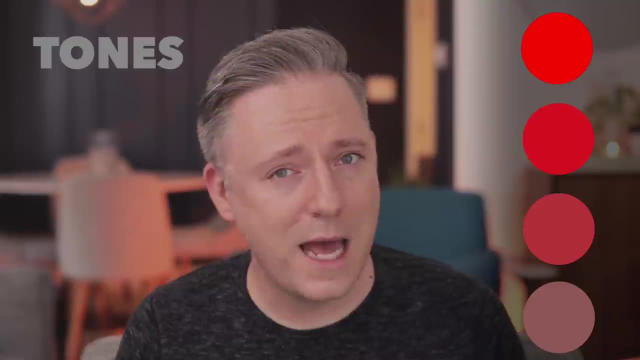 is they just become more desaturated. They just become um less like they're kind of primary bold selves and they start to become just a little bit more toned down. That's probably where we got that from. So they look a lot more desaturated, and tones are really important because these colors can look really beautiful in your space. They'll always have different undertones of the primary color, but by adding gray to that primary sort of pigment you're able to create something more desaturated And, honestly, in a living space it's going to probably look a lot. 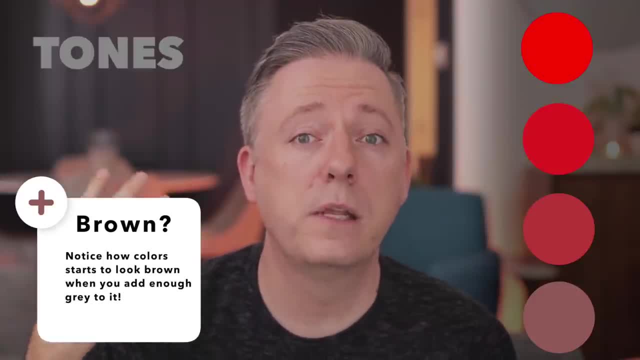 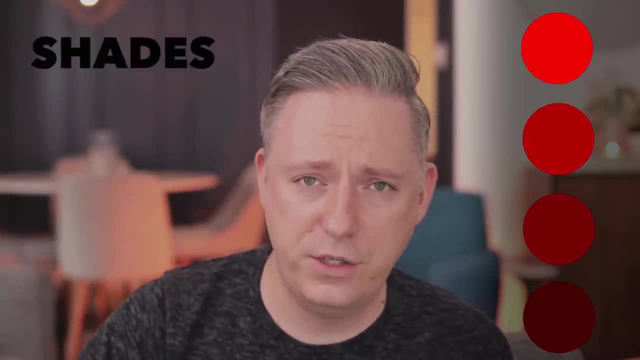 better on your walls or your furniture than if you may were to use those really, really bright colors, Right? And the third one that I want to talk about is called shades, And you've probably heard of what that one is, And that is when you add black to these different colors. So if you 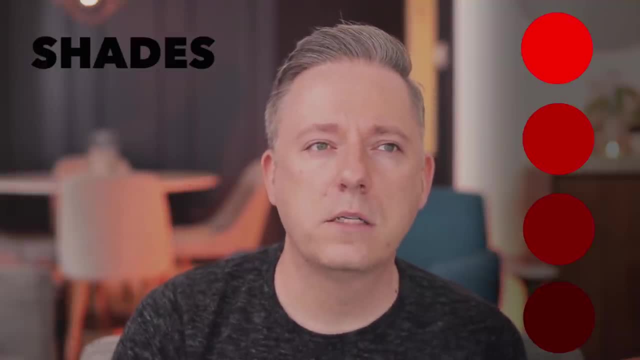 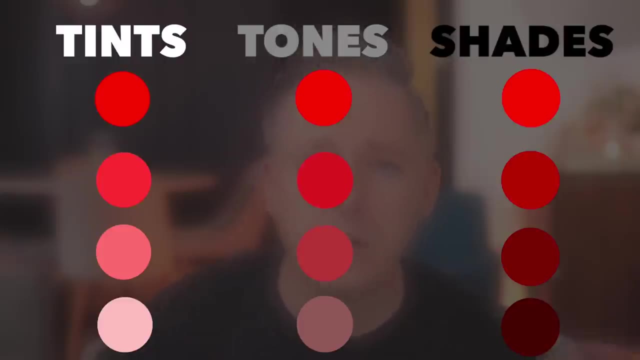 take a color like green and you start adding black to it, um, it'll start to get a lot richer and a lot darker. So that's tints, tones and shades. So when we're talking about the different color palettes, we're going to be talking about the different color schemes and combinations that 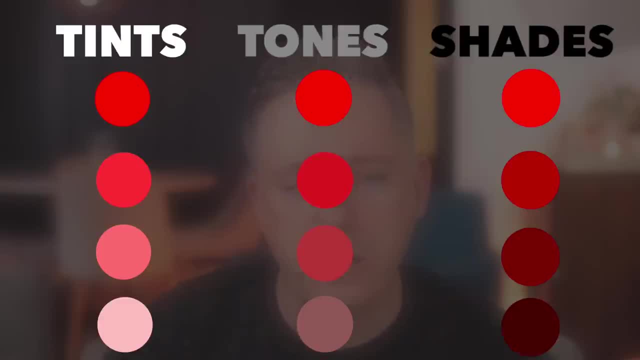 you can go through, But I really think it's crucial to understand that we don't just mean adding these primary colors together. We're talking about all the tints, tones and shades that exist within that color wheel. So when you look at it from that perspective and you look 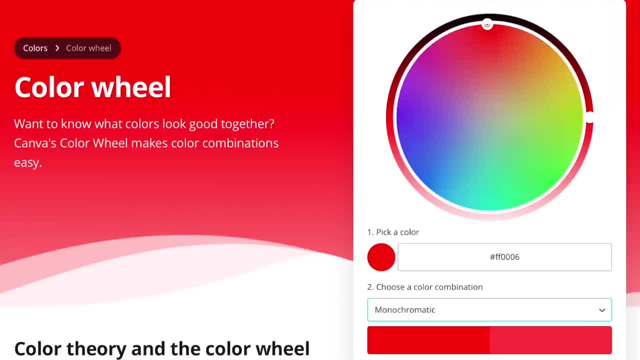 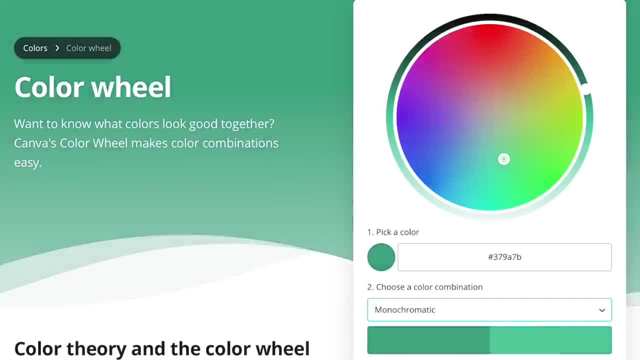 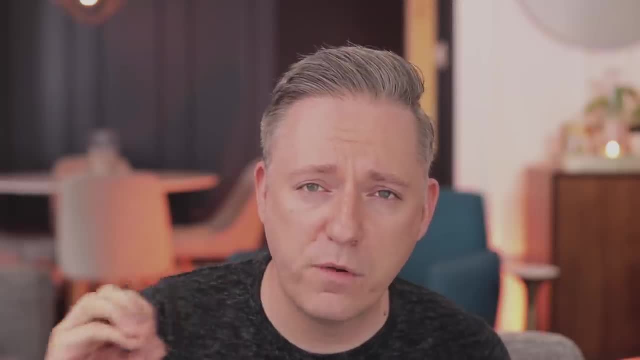 choose from. I feel like people sort of go like: oh, blue and orange, Okay, That might work, but there's actually thousands of different colors that exist within those two colors, So that's really important to understand as we move on to creating a palette. 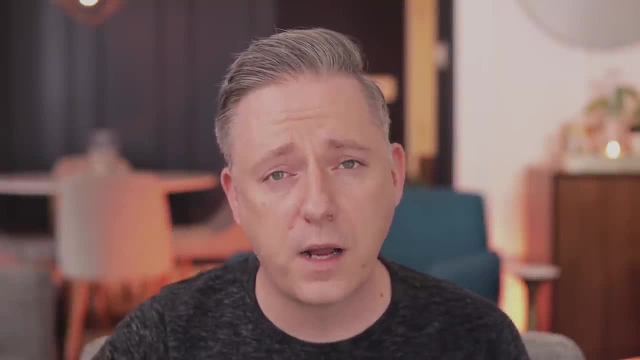 that's going to work for your place. Okay, So now moving on to different color palettes. So you have a few different options here. There are other options, but I'm going to stick to the three primary ones. So I'm going to stick to the three primary ones. So I'm going to stick to the 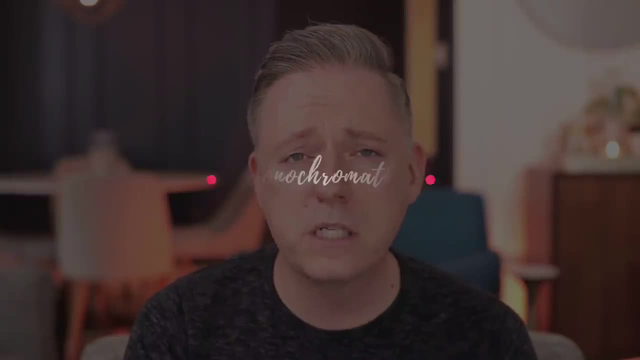 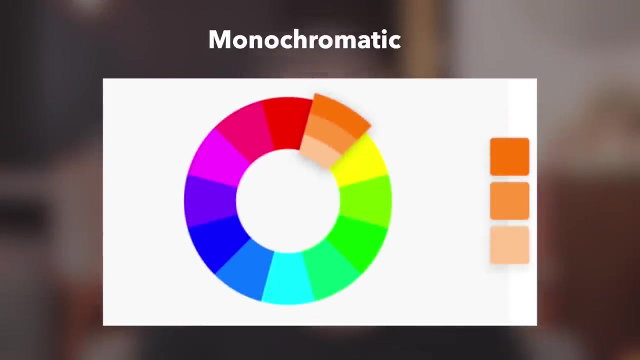 three primary ones. So the first one to talk about is monochromatic. Monochromatic just means taking one of those different slices of pie and just basically working with all the tints, tones and shades that exist in that color. So if you want to create a monochromatic blue space, 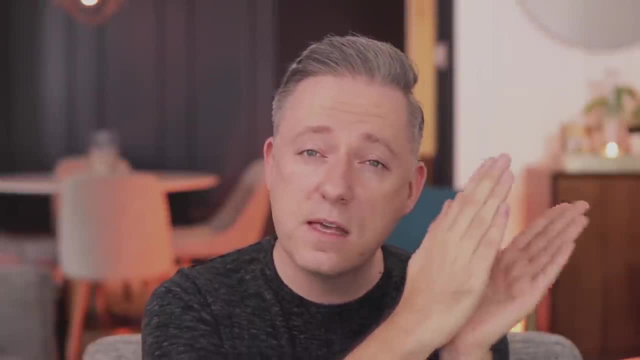 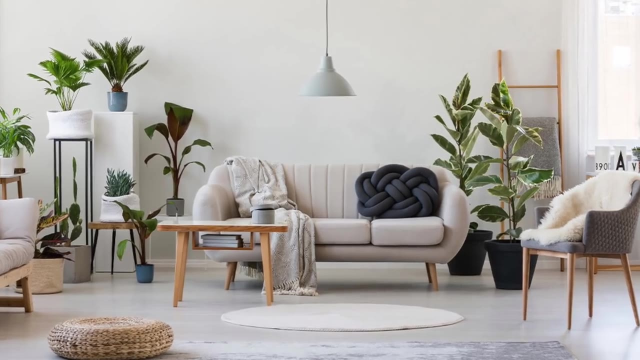 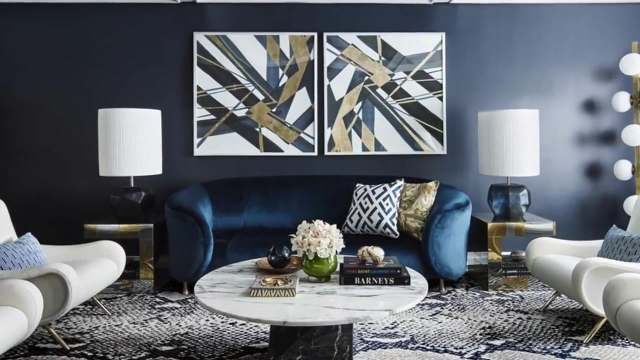 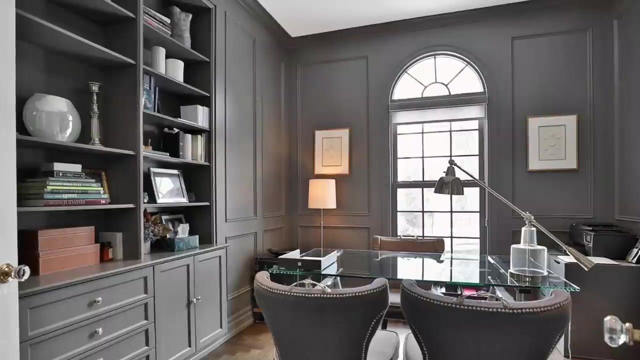 that would mean you're working with every different color that exists within this little slice of blue to be able to create for your space. Monochromatic schemes can be really beautiful, really purposeful, and let's look at some really great examples. So the second type of color palette I want to talk about is called analogous, And that means that. 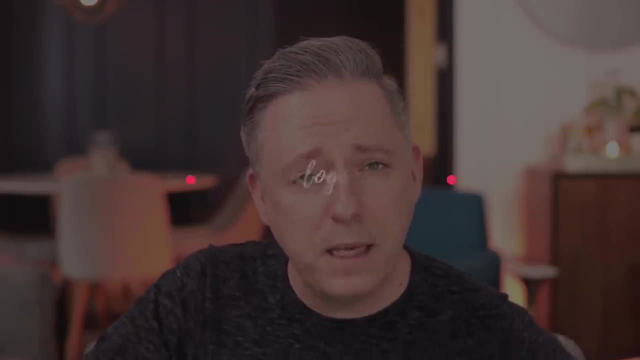 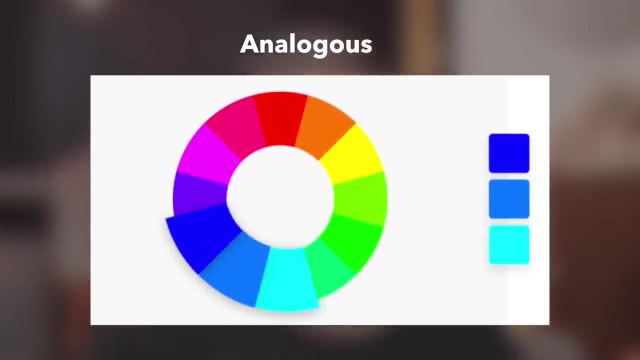 you're looking at two or three different slices of the pie of the color wheel that sit next to each other. So you know these ones work together because they sit next to each other on the color wheel. So, for example, if you were wanting to design a red, orange and yellow space, you'd be 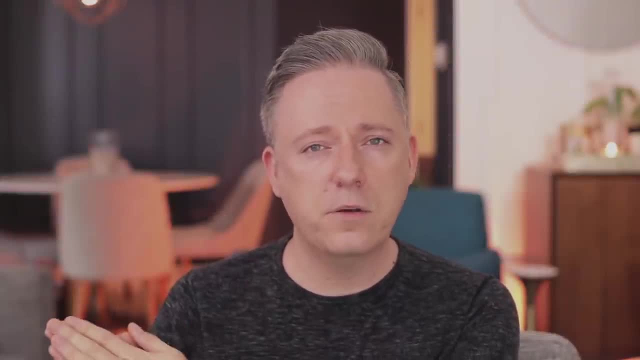 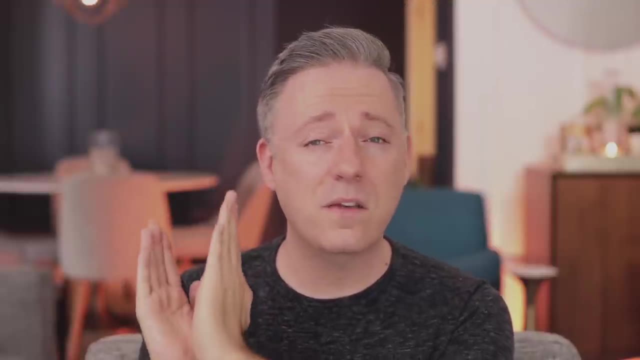 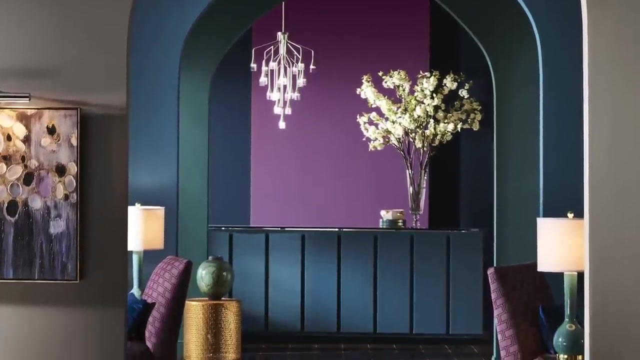 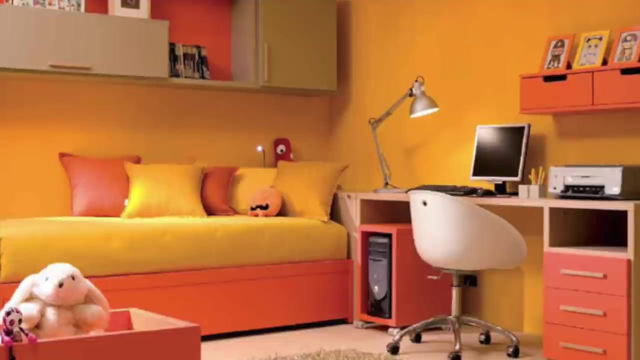 working with all the tints, tones and shades that exist within that color wheel. So you want to get all of those colors together. So that's going to be a really good example of what you're going to be working with. And then the third type of color scheme, which is, in many ways, probably one of my 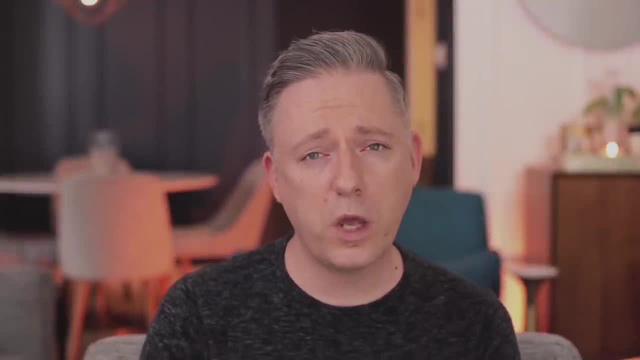 favorites, and that is a complementary color scheme. So this is working with again all the tints, tones and shades that exist on two or three different pieces of the color wheel. And then the third type of color scheme, which is in many ways probably one of my favorites, and that is a 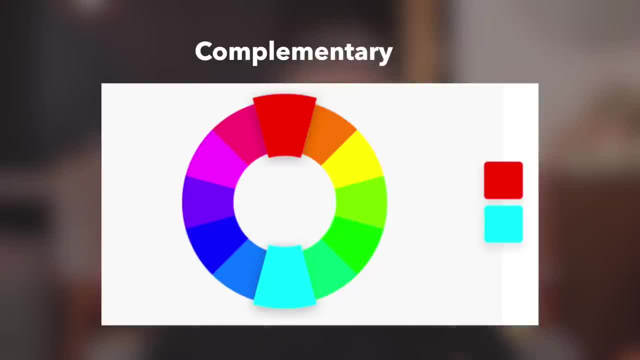 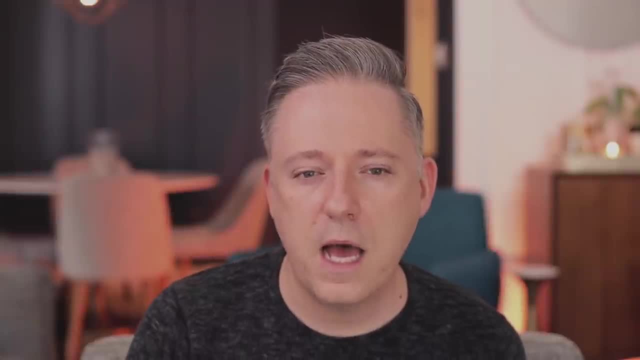 two colors that are opposite each other on the color wheel. So this is really great. for a couple of reasons I love this. first of all because there's a certain contrast that comes with using a complementary color scheme that you just don't necessarily get as much from analogous or 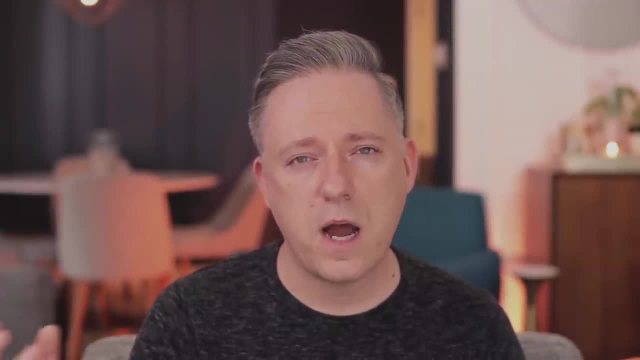 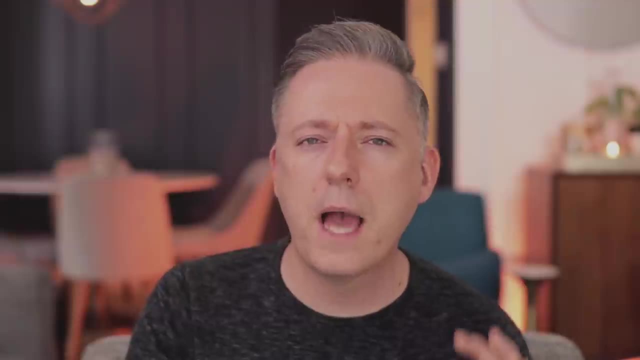 from a monochromatic scheme. So you're definitely getting a lot of contrast, which is kind of creating sort of visual appeal from these two colors that exist opposite each other. And the second reason is that it's a really great way to combine warm and cool colors on. 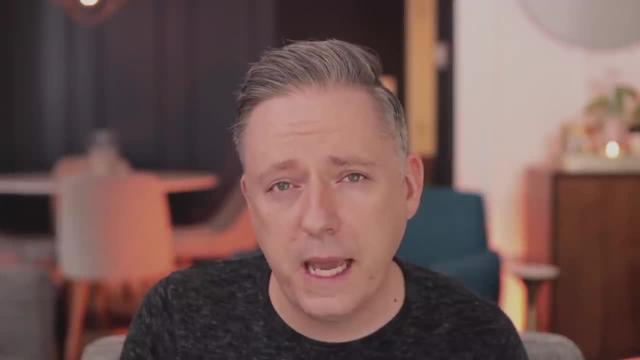 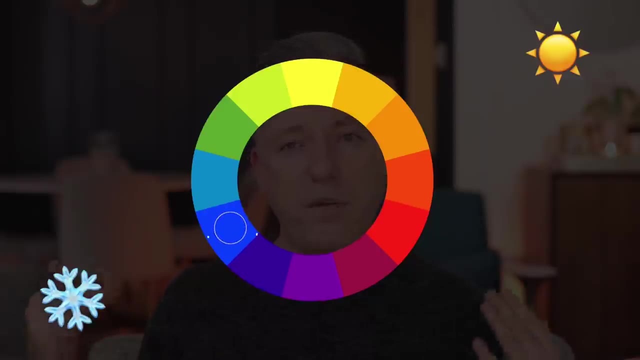 the color wheel. So that was a question I got a lot on my. How to Choose a Neutral Paint is when we're trying to combine these other two undertones. what people get confused is what if I have undertones of blue and I have undertones of orange, for example? Well, here's the good news. 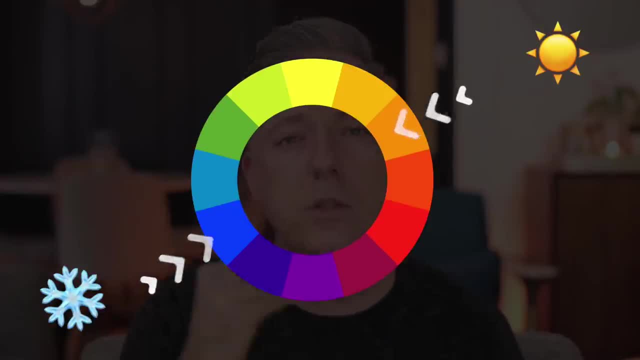 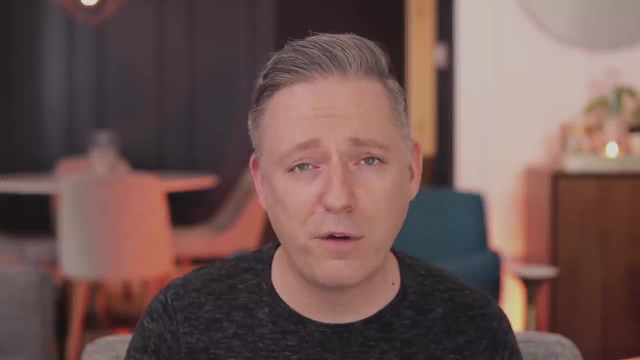 blue and orange sit opposite each other on the color wheel. So if you're able to reinforce the different colors from these two different sections of the color wheel, you're going to create something really cohesive and really beautiful, And I'm going to go into more detail on that. 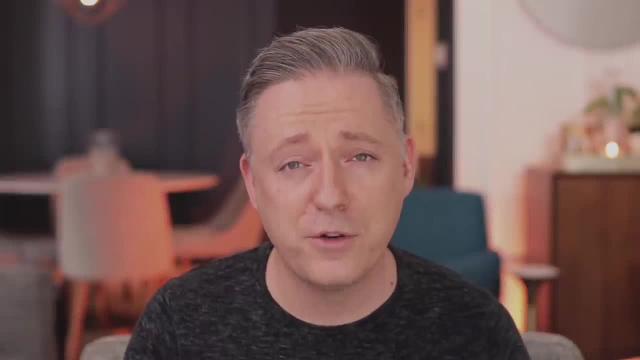 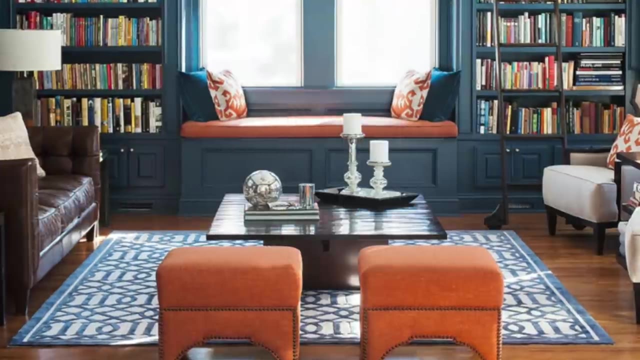 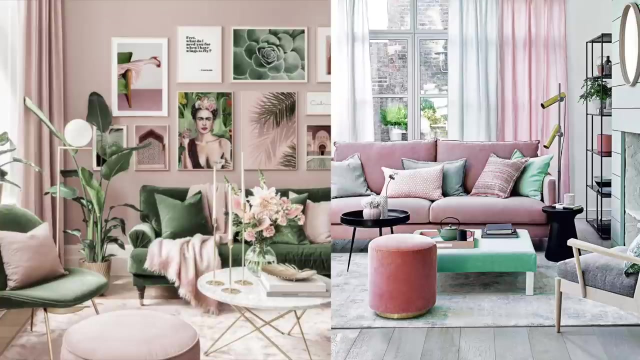 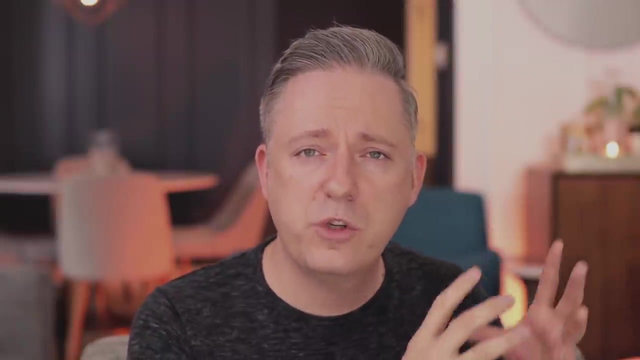 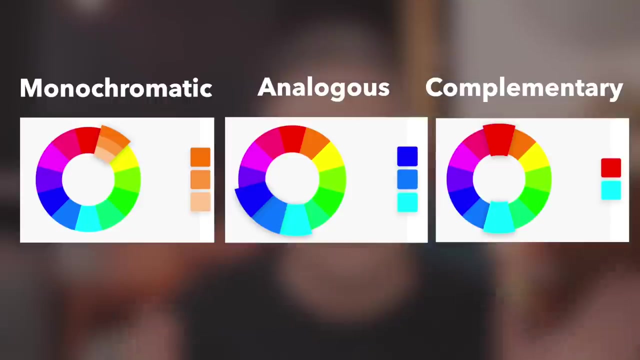 in a second, But first let's look at some gorgeous examples of complementary color schemes. Okay, so we understand that there are different tints, tones and shades within each color. We also understand that there's different ways that you can build a color palette that's going to work for you. Now that we've decided that, let's talk about the. 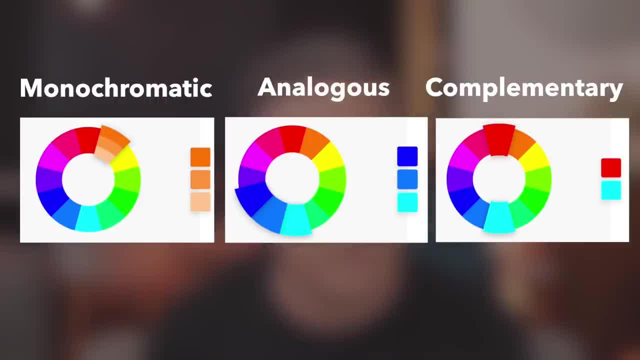 third way, which is how do you combine them in a really cohesive way? And the good news there is that there is a lot of different ways that you can build a color palette that's going to work for you. So here's another example. this is a design principle called rhythm- All that rhythm really means. 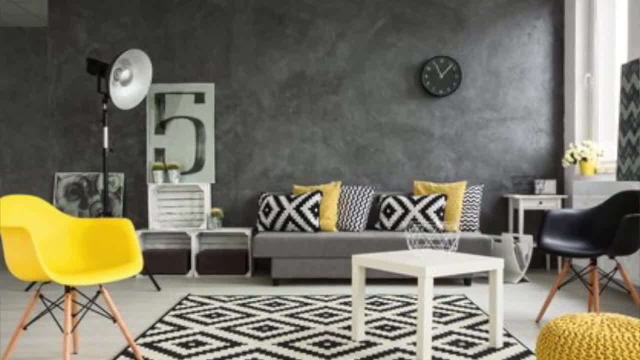 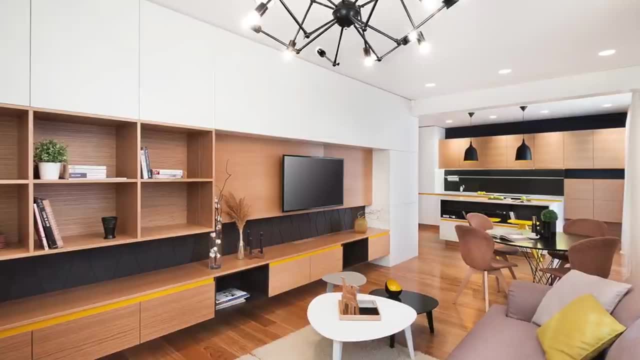 is that when you start to repeat shapes and color and pattern and texture throughout a space, it makes them look cohesive and work together, And color is one of the easiest ways for you to do this. So, now that you've picked your color scheme and you understand how they're going to, 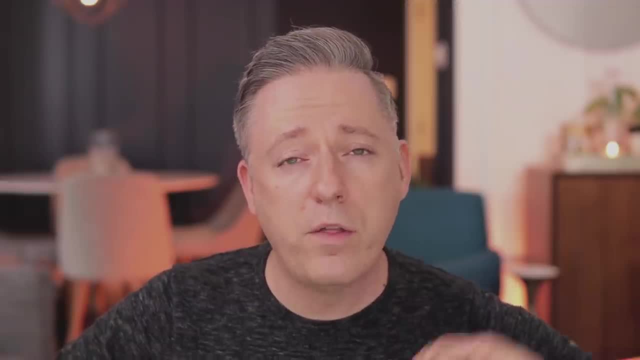 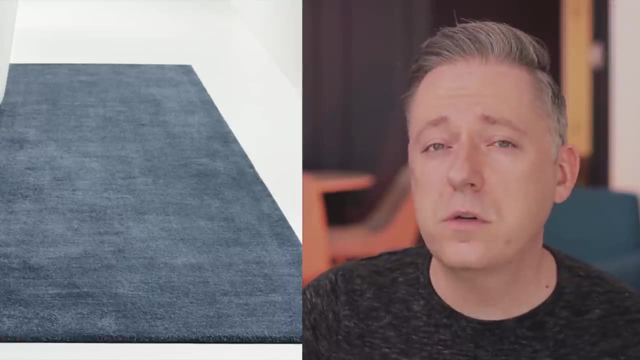 work together, then all you need to do is start to really repeat them, Whether that means in really obvious ways, like a blue throw in a blue pillow and a blue vase, or it could be in undertones that you're using, so you might use a white paint on the wall with a blue undertone. that ties in well. 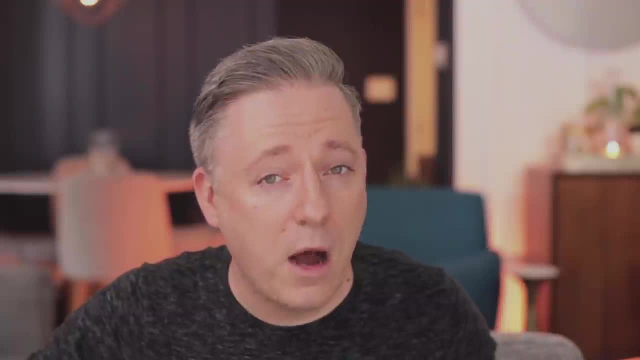 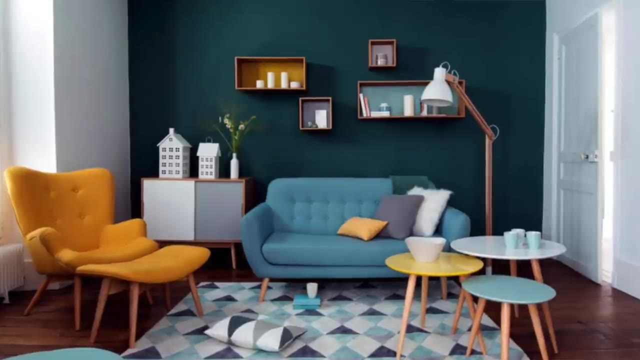 with maybe a blue rug or a blue pillow or maybe a couch that is gray but has slight blue undertones, and you can start to kind of see how you can pull these things together by repeating colors over and over in the space. and it's that consistency, it's those different patterns. 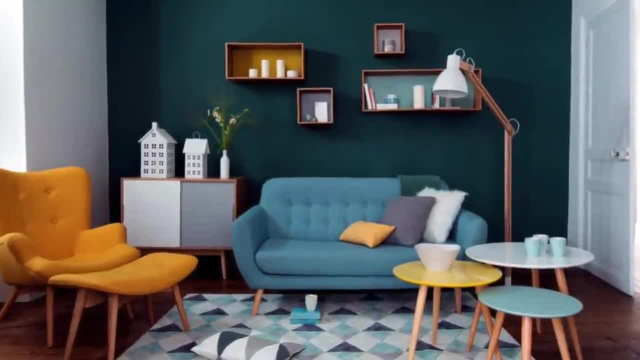 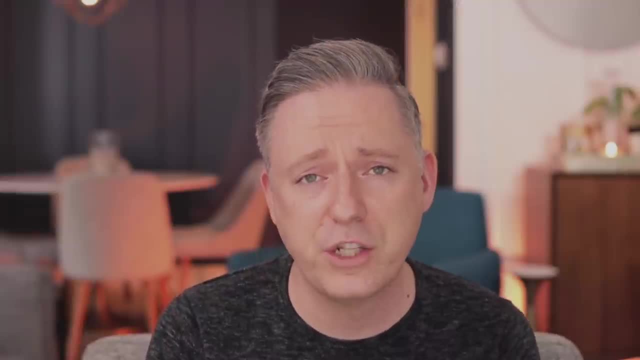 that you see over and over in a space that visually pulls the space together and makes every little thing sort of feel like it belongs there. okay, so now practically let's go through like a real world example of how i can do this for you, so you can see how i would do it and maybe you 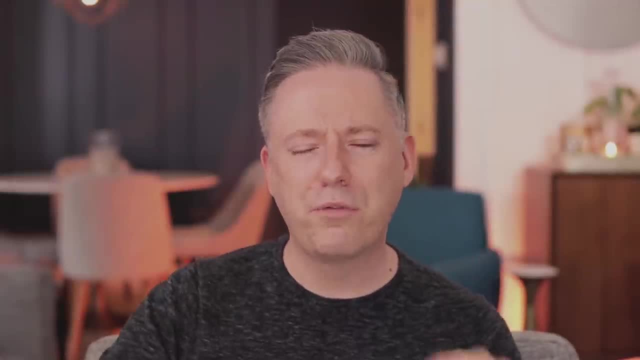 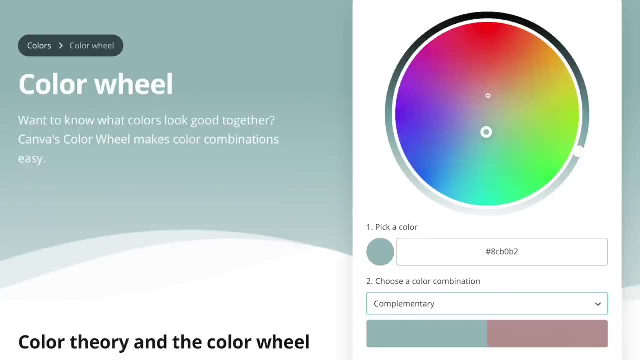 can learn, but what would work for you? so one of the first things i would do- a great resource that i think is an awesome color wheel- is on the website canva. i'll link it down in the description. but what canva's done is they've got- and there's a few that are out there. i just kind of like this. 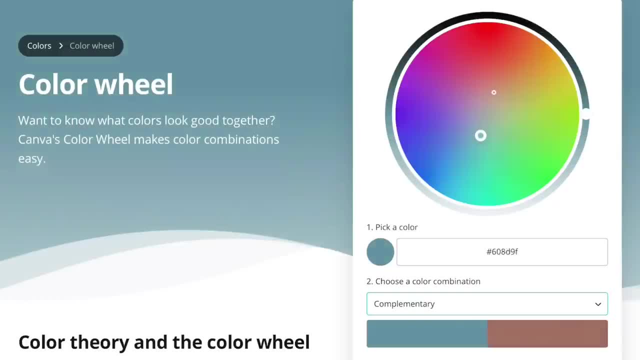 tool um is that you're able to use the three different types of color schemes that we talked about. then what you can do is you can pick a color on the color wheel and you can start to see which ones are opposite, which ones are complementary. it'll also give you different examples. 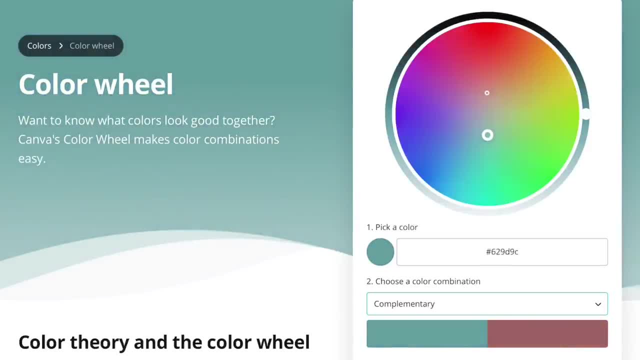 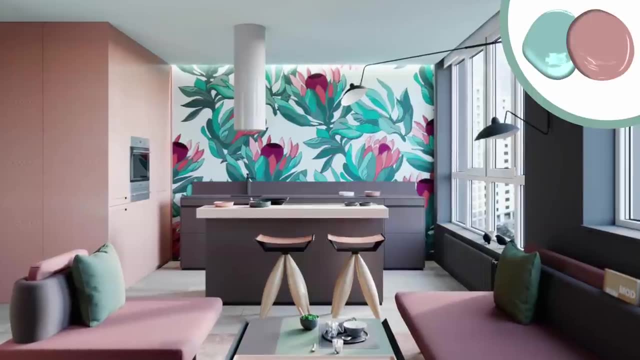 in a monochromatic or an analogous color scheme that are going to work really well for your space. and this is like an awesome jumping off point for you to be able to start to pull in different things when you're shopping or when you're pulling in samples to see what's going to work for your